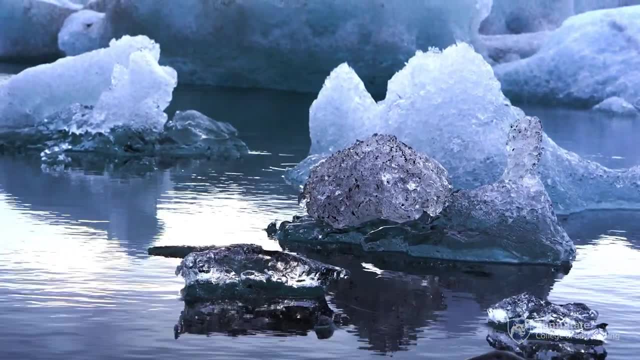 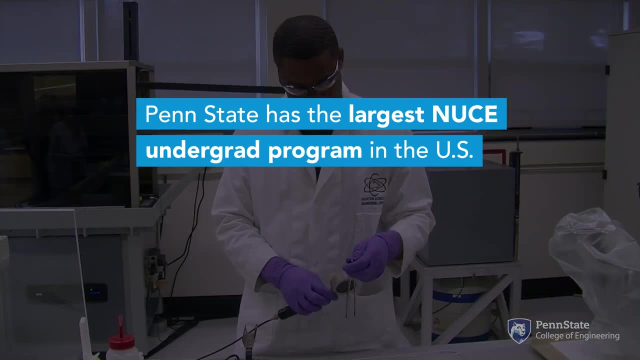 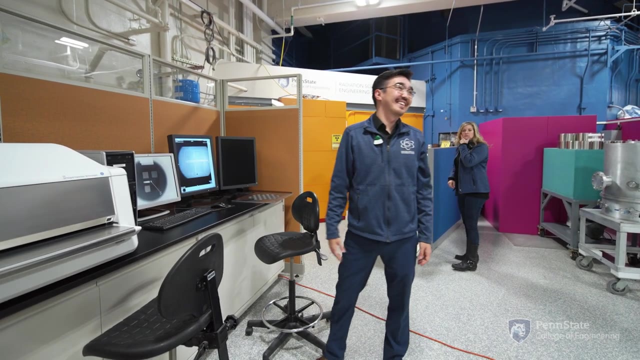 for sustainability and to address climate changes as a carbon-free energy source. Many go on to graduate school, after which they work in academia, industry or at research laboratories. Penn State's Ken and Mary Alice Lindquist Department of Nuclear Engineering collaborates with the Brazil Nuclear Reactor, the longest operating licensed. 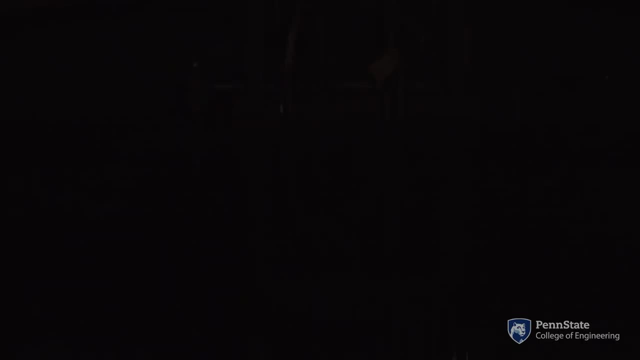 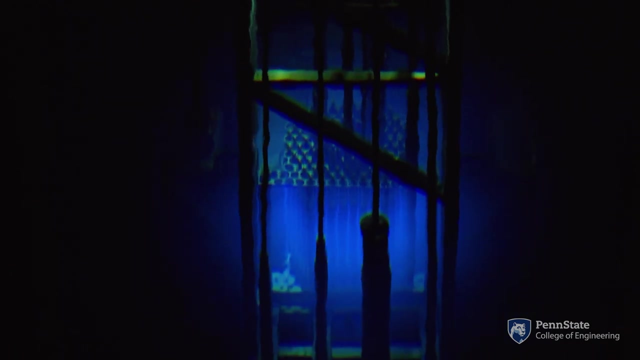 research reactor in the country. Faculty and students alike use this reactor to conduct research that propels the field forward, including the use of neutron science in materials and life science research. One of the reasons Penn State is a great place to come for nuclear engineering is the Brazil. 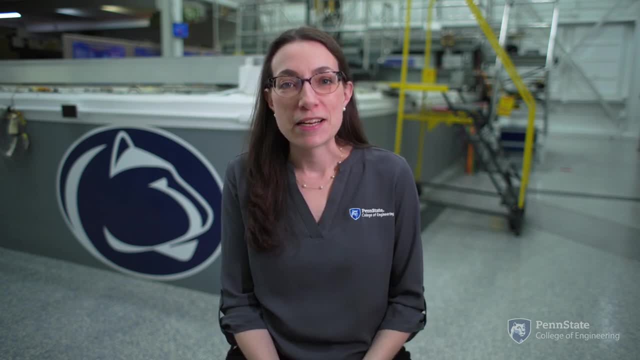 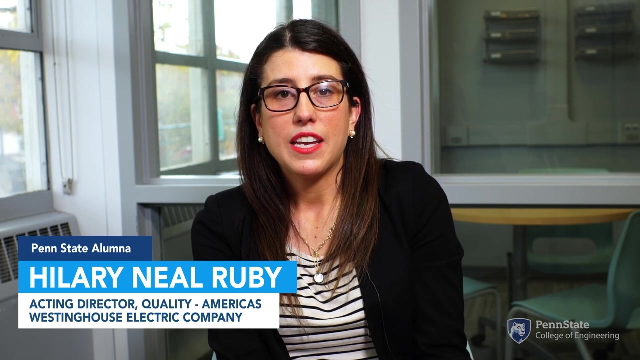 Nuclear Reactor right behind me. This reactor is a national resource, and students can have the opportunity to become operators, but also to use the neutrons that the reactor produces as a part of research. What I love about being a nuclear engineer is just the opportunity to interact with people. 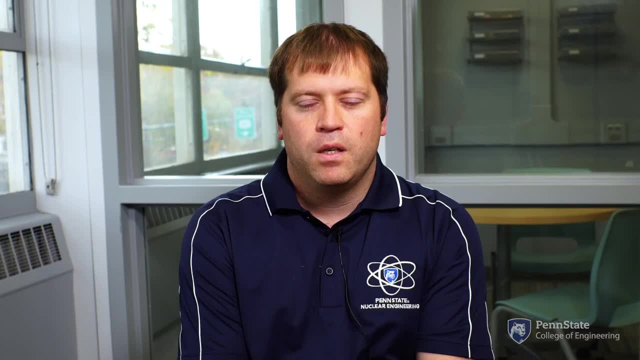 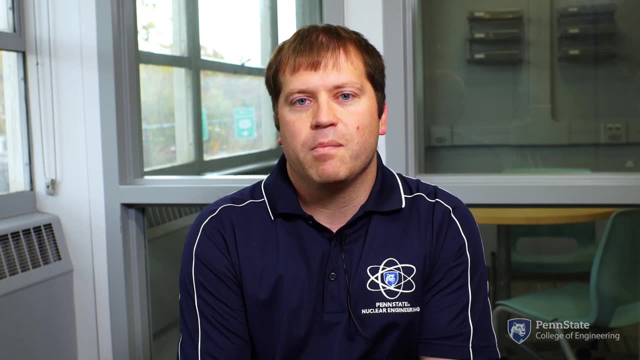 to solve problems and to really work in a global context. The nuclear engineering field is growing pretty rapidly. It used to only be a power engineering field, but now we have a lot of ties into medicine materials labs and other places. 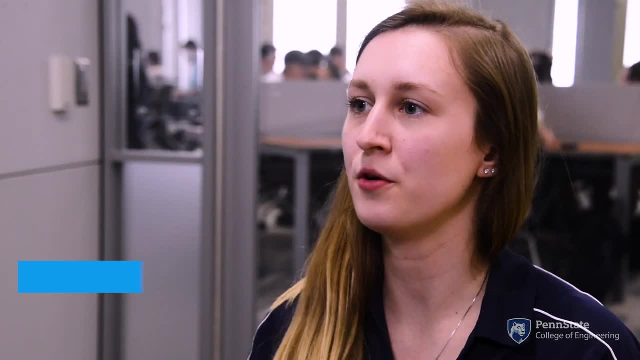 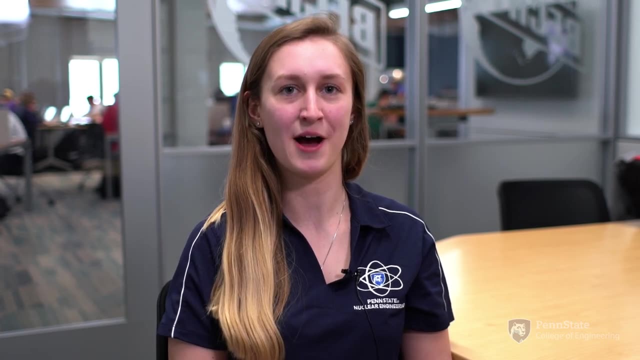 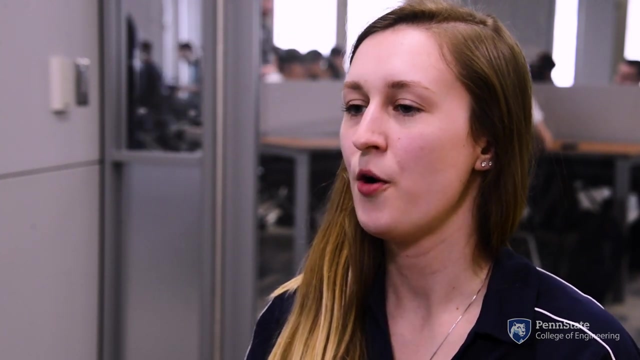 even propulsion. as the space industry starts to come back, I kind of knew I always wanted to be in STEM. I saw The Incredible Hulk got hooked, saw Iron Man and Iron Man became my favorite And I did a little bit of research and found out that his arc reactor that powers his suit. 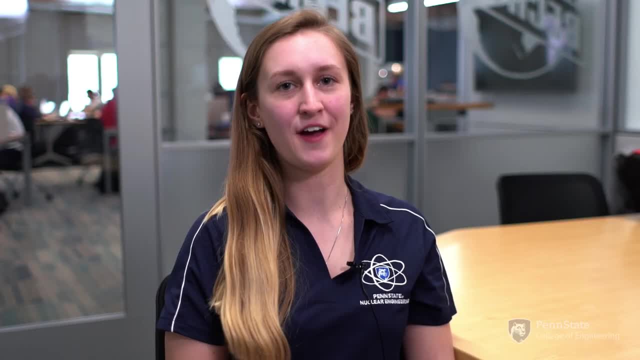 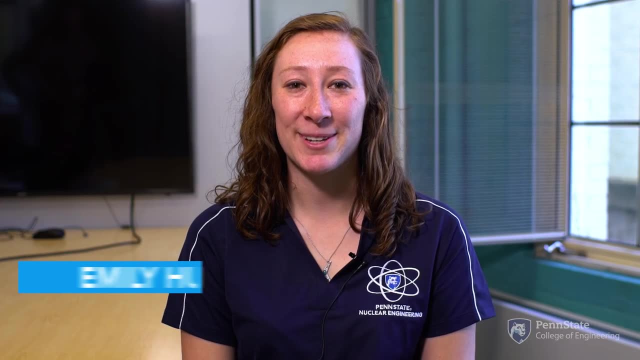 was basically a nuclear reactor. So I was like: I want to build the Iron Man suit, I'm going to become a nuclear engineer, and here I am. One of the aspects I love most about being a nuclear engineer here at Penn State is that 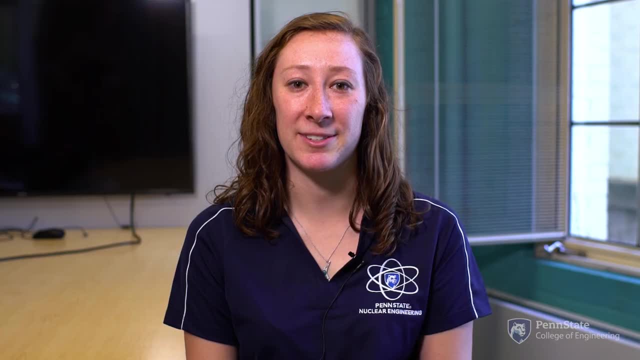 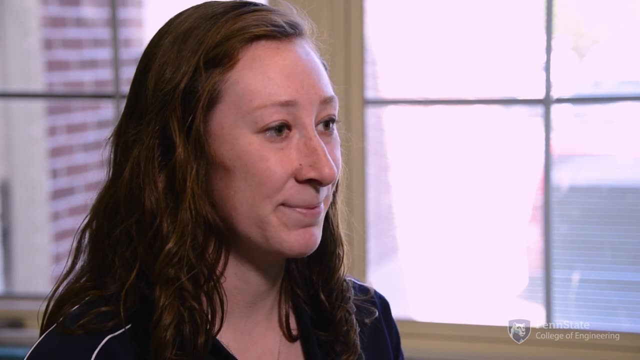 our class sizes are typically smaller than most larger engineer classes, So you really get to know everyone in your major on a one-to-one basis and you make all these meaningful connections. There are a lot of research for undergrads in nuclear engineering. So if you talk to, 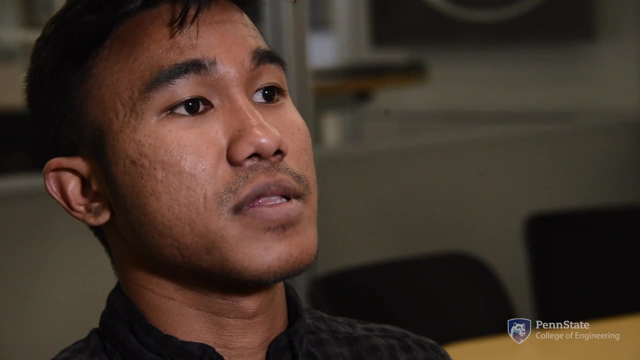 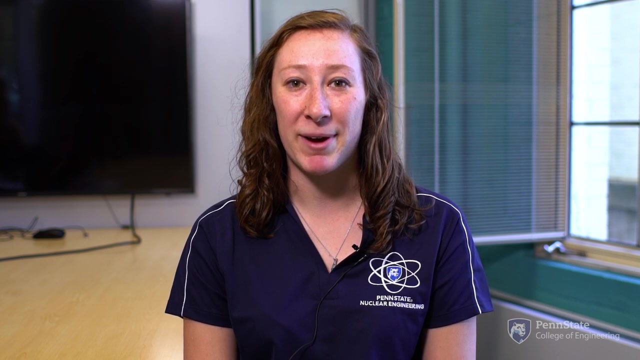 your professor and you hand in your resume, they would more likely to accept you doing your research As a nuclear engineering student. you can actually have the opportunity to work part-time at the reactor on campus. You can become an auxiliary operator so you can help prepare.